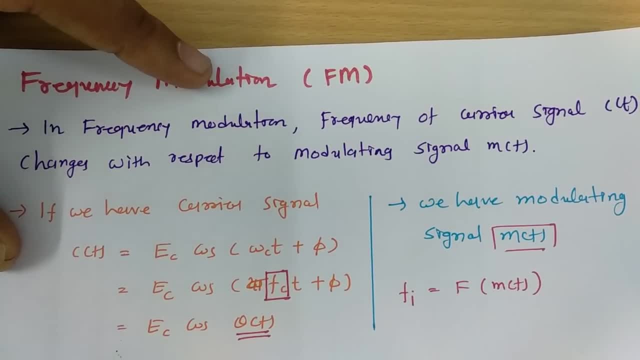 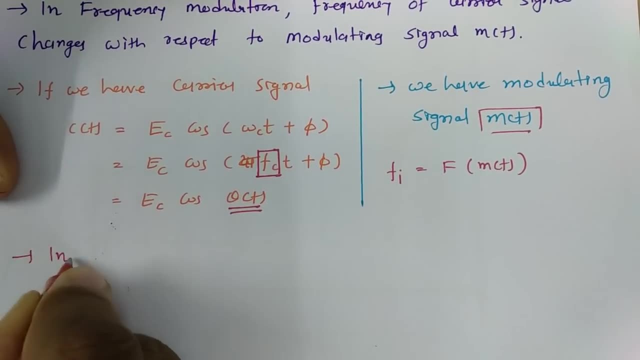 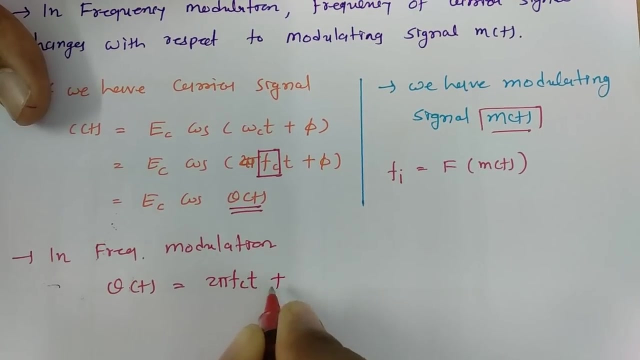 Now how this function is there. that is what I will be discussing over here. Then after we will design frequency modulator. So basically in frequency modulation, this angle, theta t, that is what having change in this carrier frequency. So how that will change, see theta t. now that will be 2 pi fc t plus there will be change in frequency. 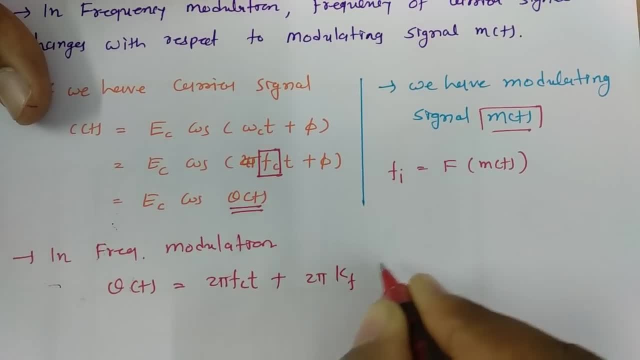 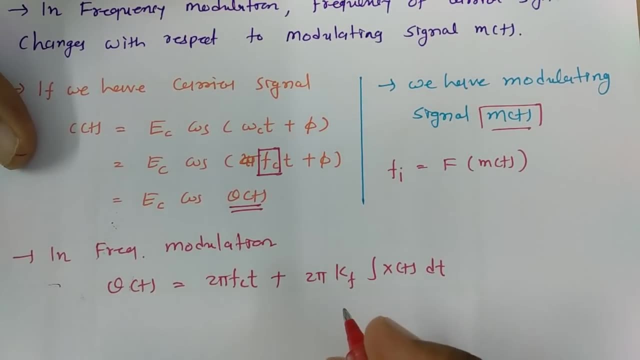 So that will be 2 pi fc, t plus there will be change in frequency, So 2 pi kf into integration xt, dt. So here we can understand like: see this xt, that is what varying from 0 to t. So based on this modulating signal, that resultant frequency is getting deviated. 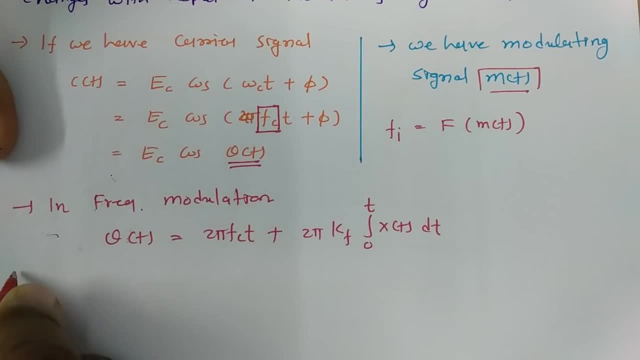 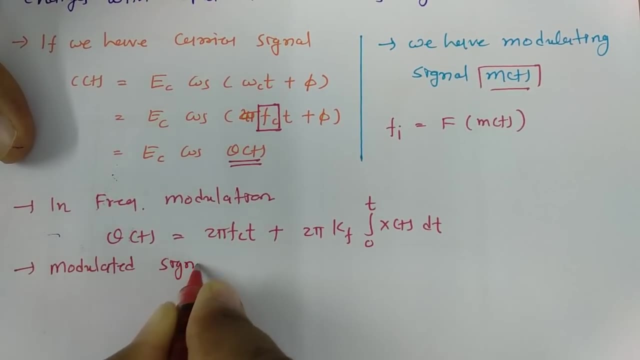 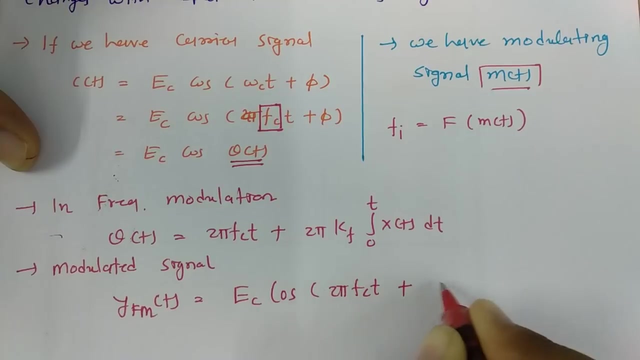 So our frequency modulation will be modulated signal will be: That will be y of fm, so that you will be finding ec where magnitude of carrier signal is not changing, only frequency of carrier signal is changing. So that will be ec cos of 2 pi fc t plus 2 pi kf, integration 0 to t xt dt. 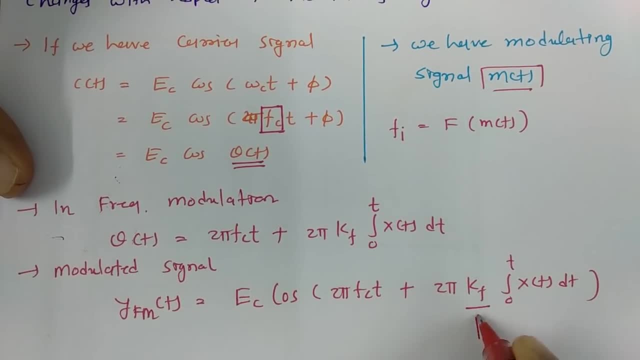 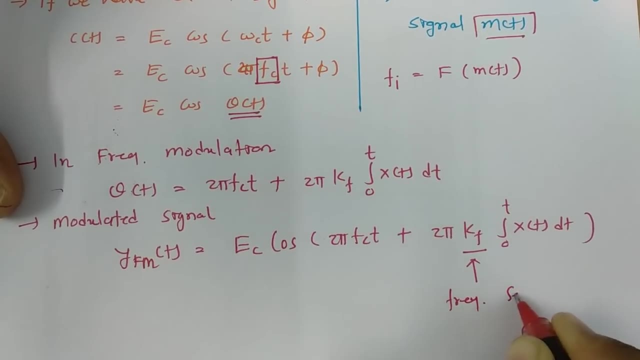 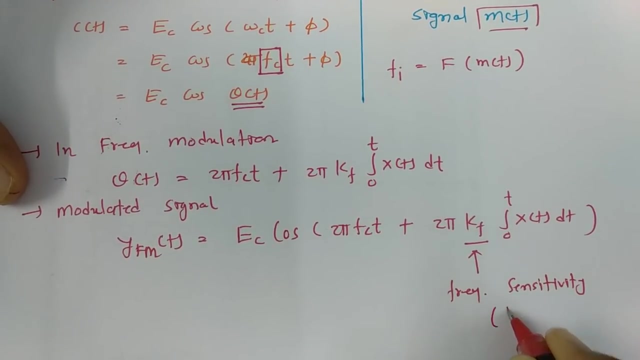 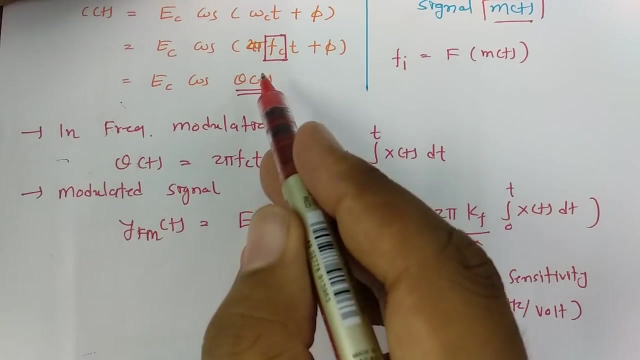 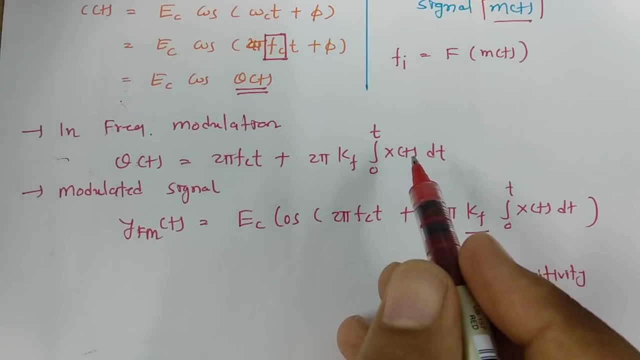 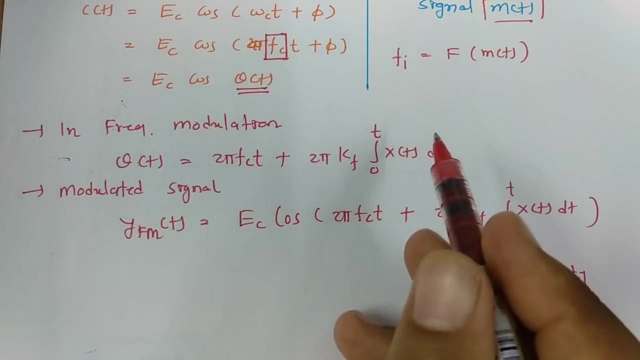 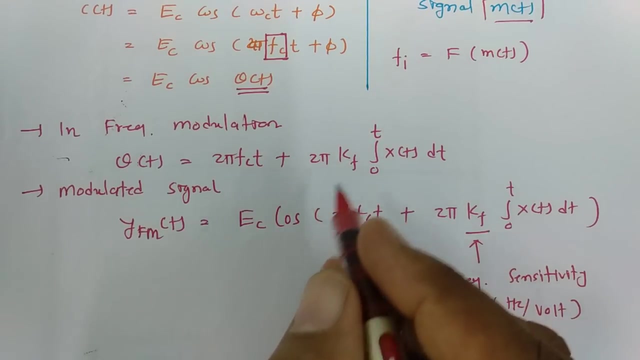 Now here this kf, that is frequency sensitivity, it is frequency sensitivity and its unit that is there in terms of hertz per voltage. So basically, in frequency modulation, frequency of carrier signal that changes like this, Where what we do, What we do is we take integration of xt or serval time interval, and if that interval, integration is positive, deviation of frequency is positive. and if that variation of frequency is negative, deviation of frequency, that will be negative. and here kf is frequency sensitivity and its unit is in terms of hertz per voltage. 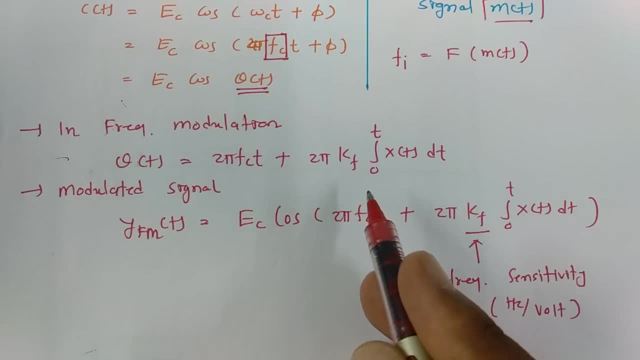 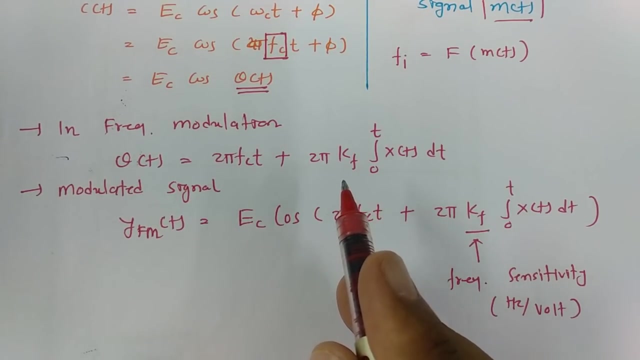 So kf justifies Sensitivity of deviation of frequency. if value of kf is high, then deviation of frequency is high, and if value of kf is low, then deviation of frequency is low. So this is what the basic thing that we need to keep in our mind when we talk about frequency modulation. 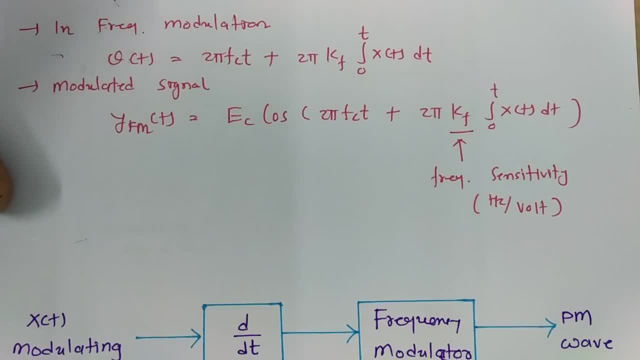 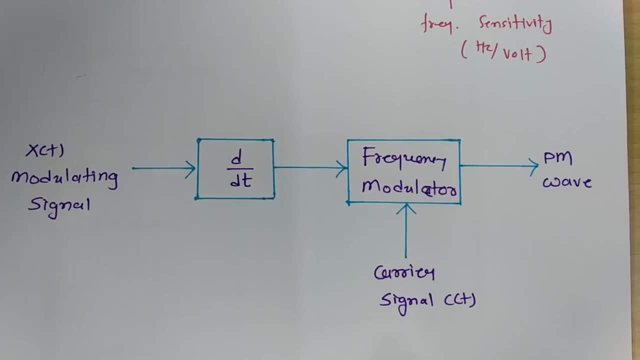 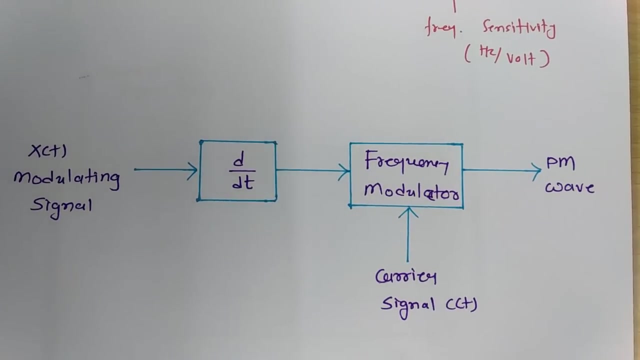 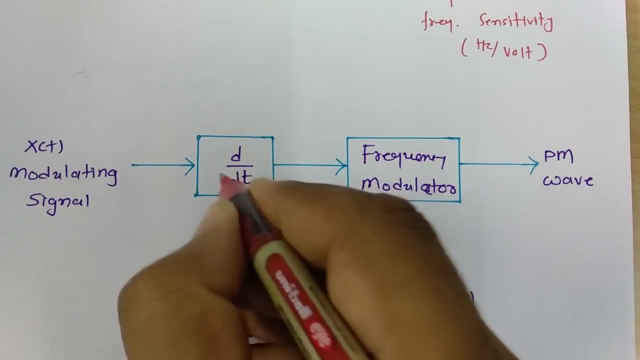 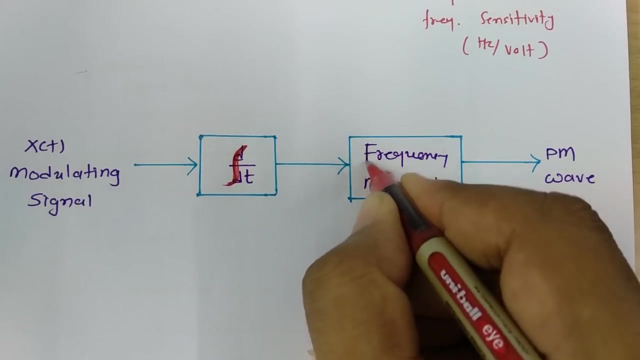 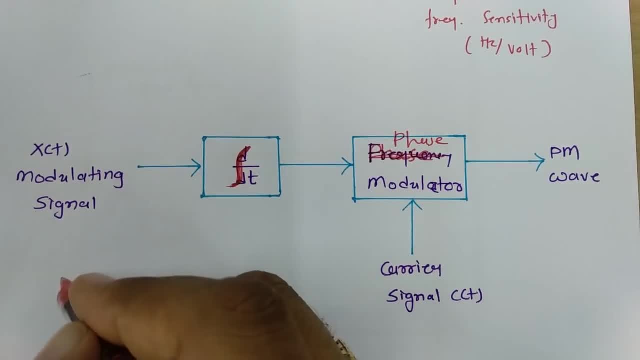 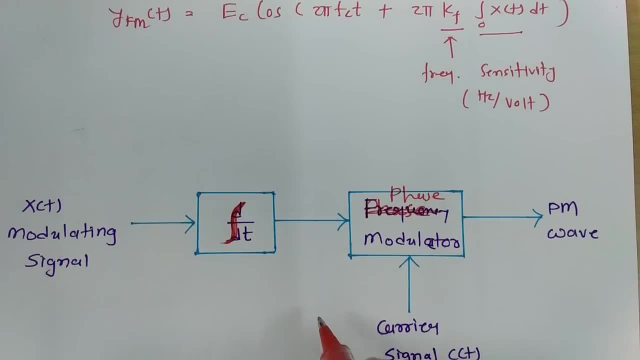 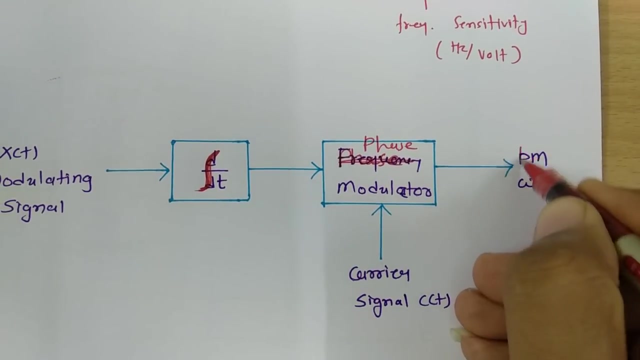 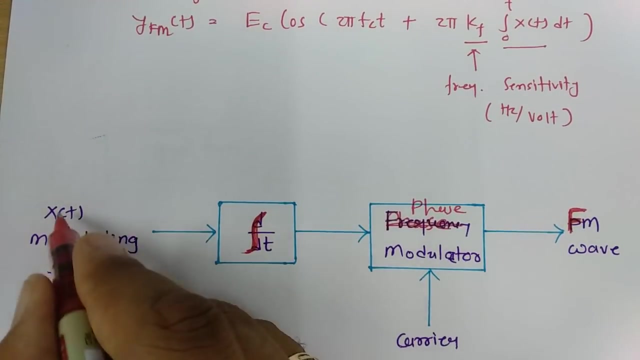 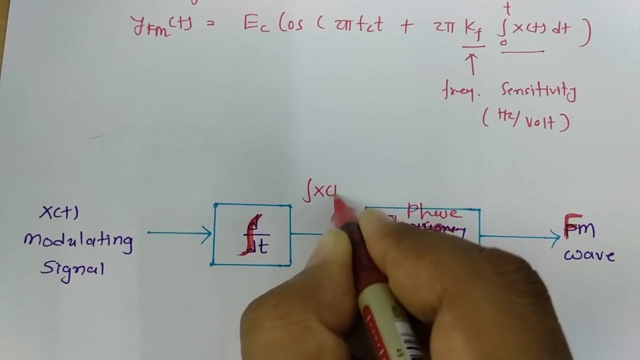 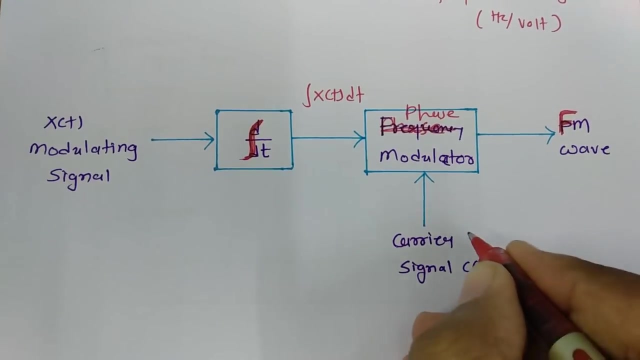 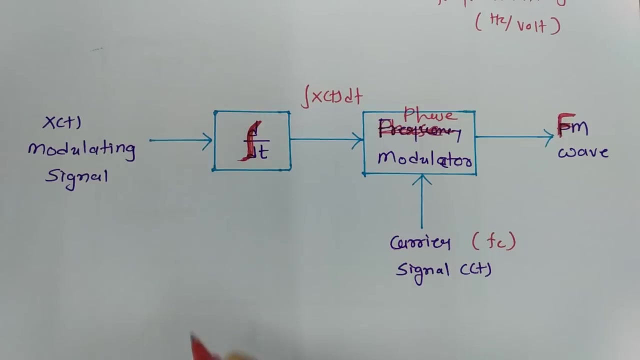 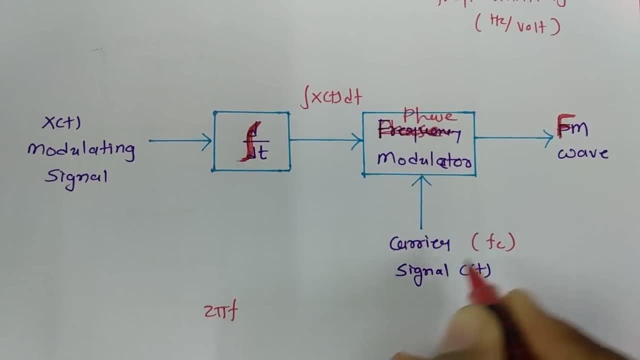 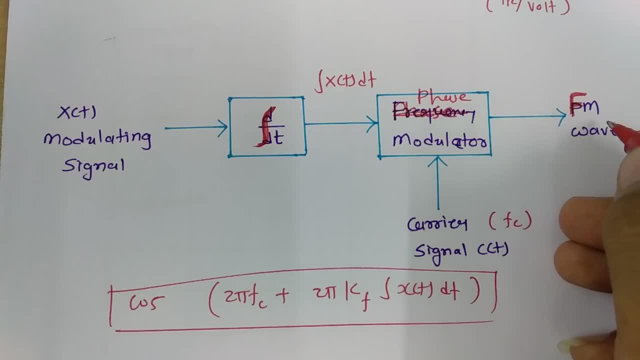 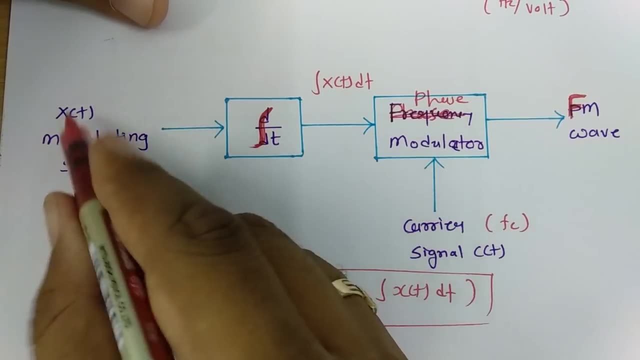 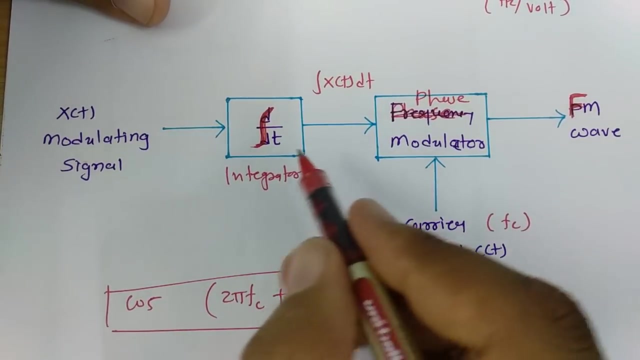 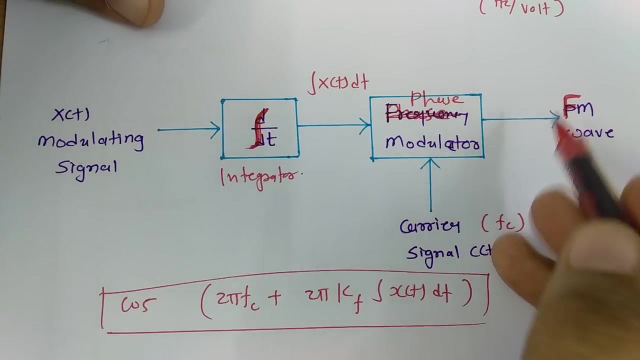 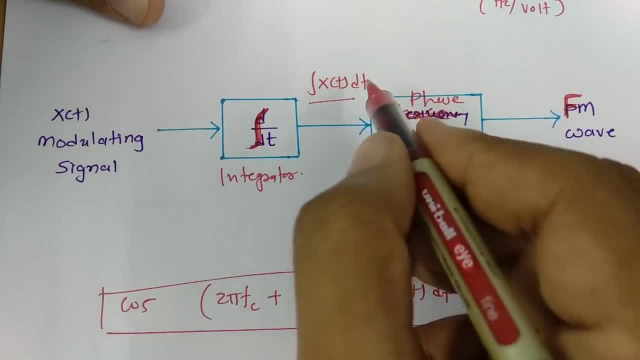 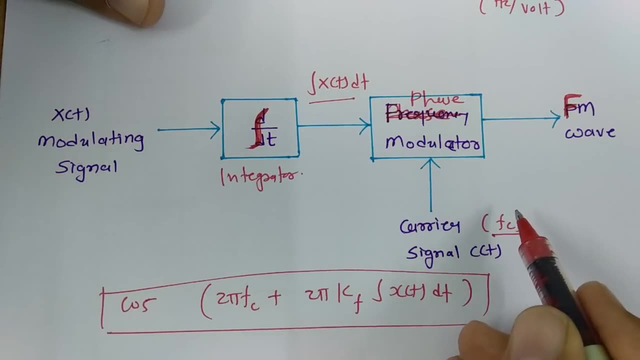 over here. carrier signal is fc and if you do phase modulation of this two, so phase modulation means phase of fc plus phase of this, so that will be fc into 2 pi plus 2 pi into this, into constant kf. that i am multiplying, which is what? frequency, sensitivity, so that is what the actual phase. 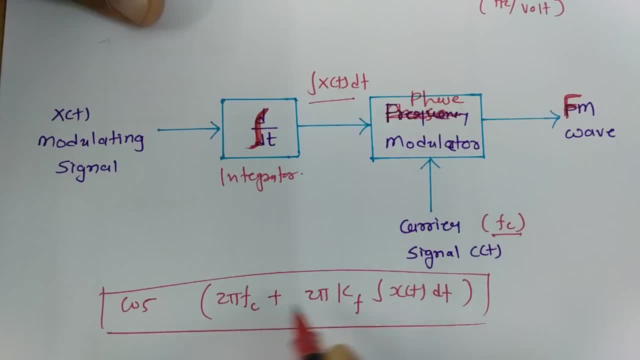 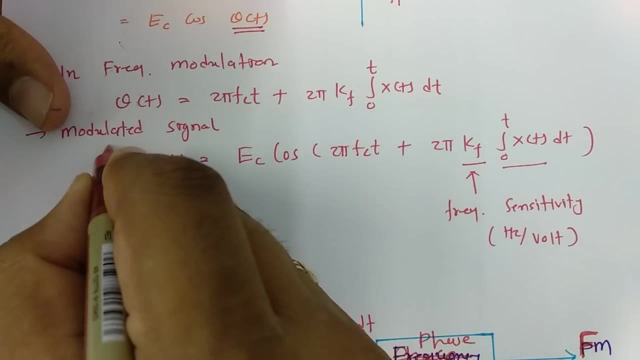 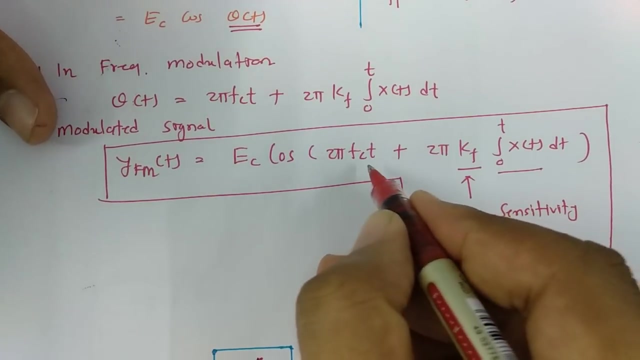 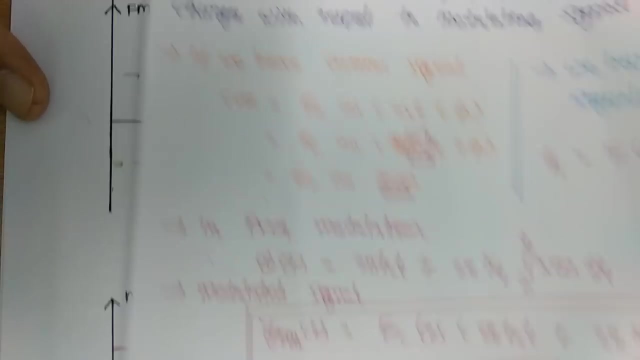 of resultant signal and that is what exactly: frequency modulated wave. so, basically, when we talk about basic formula of frequency modulation, that is this. so this is what we need to remember, where what we change is we change frequency as per this of carrier wave. now let us try to 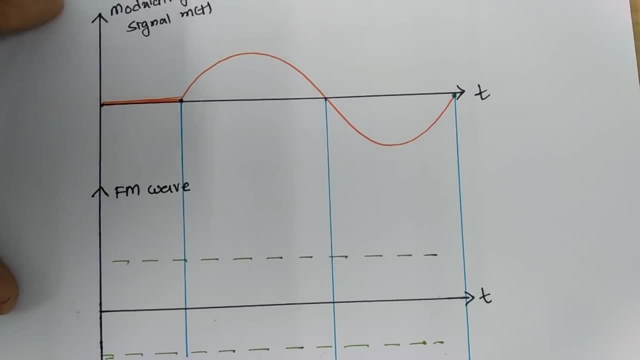 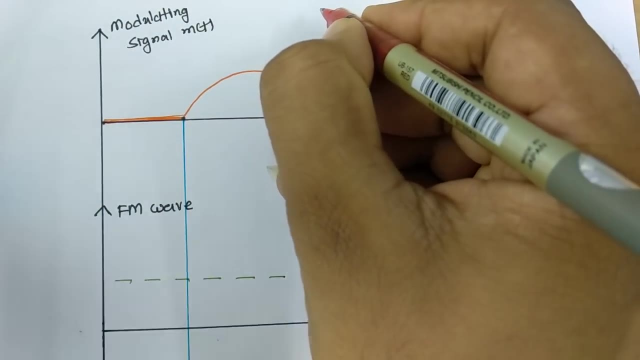 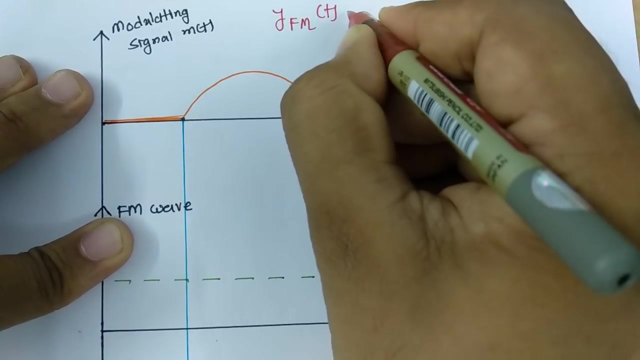 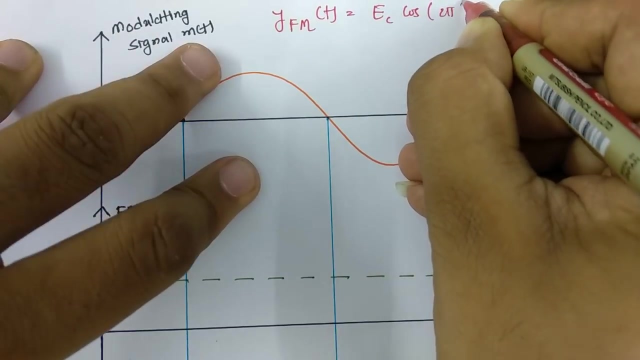 understand that with respect to waveform. so it will be more clear now. now see, as i have told you, in frequency modulation. in frequency modulation, basic equation is fm of modulated signal fm, that will be ec cos of 2 pi fc t plus 2 pi kf integration. 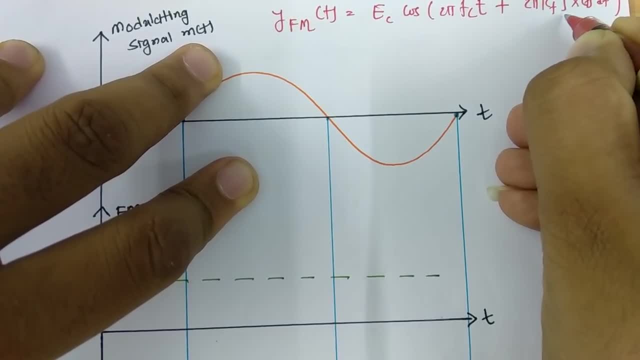 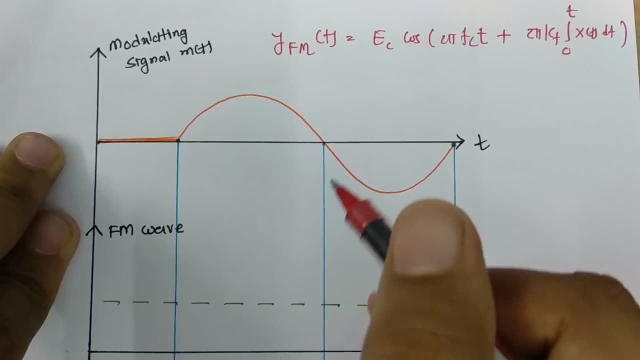 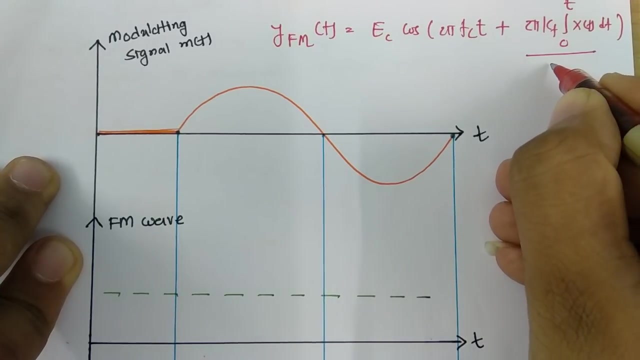 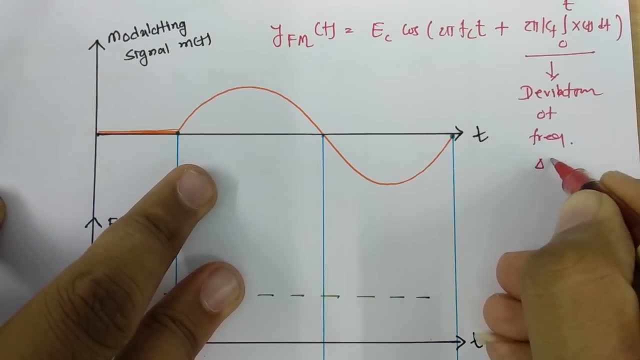 xt, dt, where integration is from zero to t. see, this is the basic equation which is there with fm, now here, if you see this term. so that explains you. deviation of frequency. now we can clearly understand: if we have positive magnitude, then deviation of frequency will be positive. and if we have this, 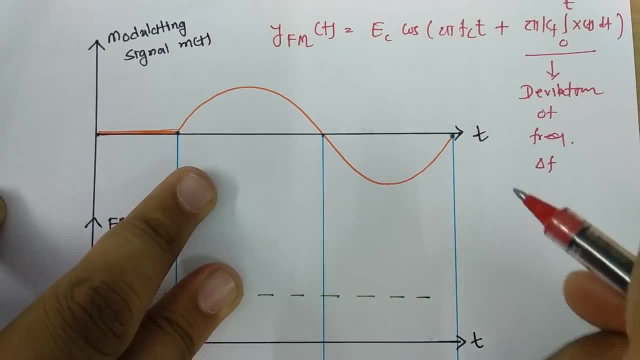 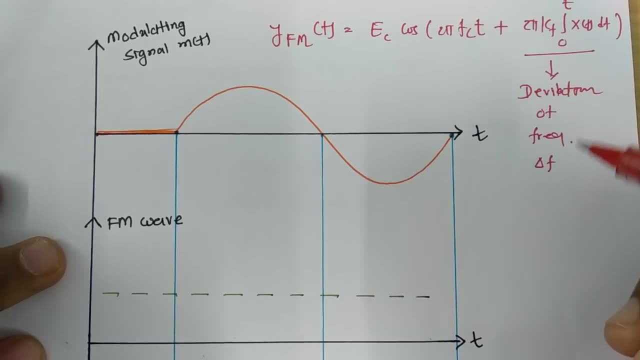 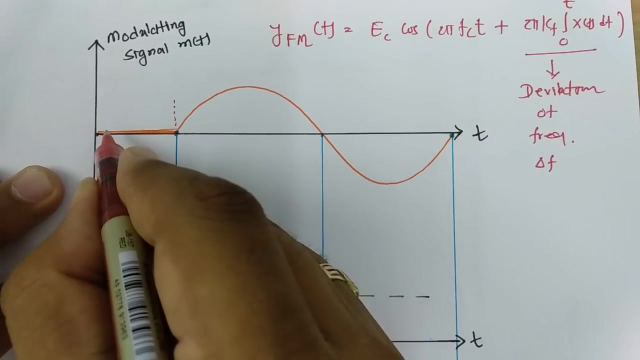 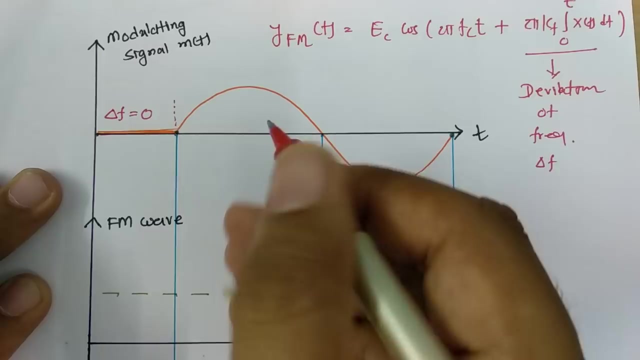 negative magnitude of this integration, then deviation of frequency will be negative. and if we have zero magnitude, then deviation of frequency will be zero. so over here we have carrier signal. one can see now here carrier signal magnitude is zero, so deviation of frequency will be negative. so we are going to find out this word properly so we will get this. so here we have positive. 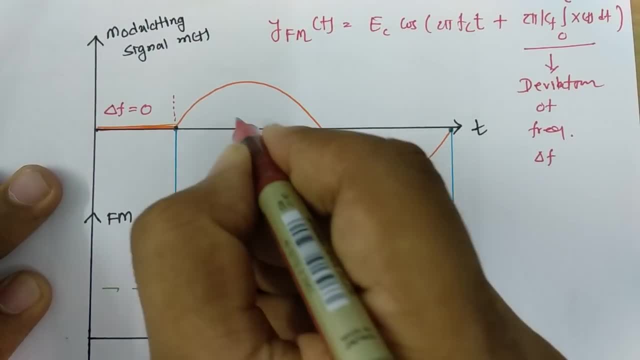 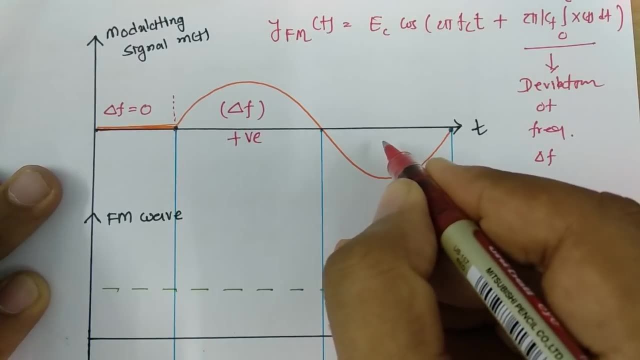 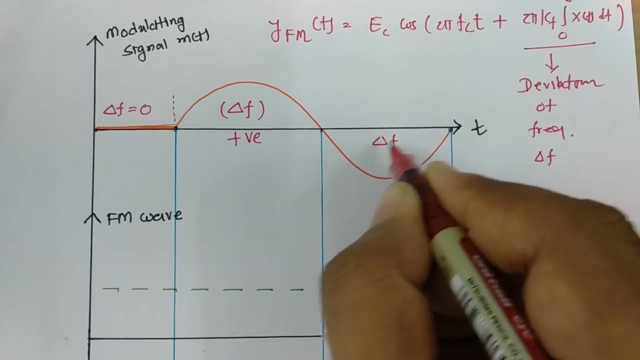 magnitude of carrier signal, which means we have positive magnitude of frequency of zero, so at this moment is 0. so at this point we can have another infinite of closing system, so we can have outside frequency of flow, so we can cove a negative magnitude of total flow. so this way we will have the 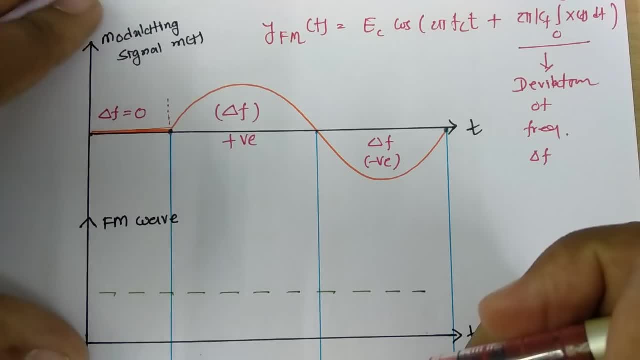 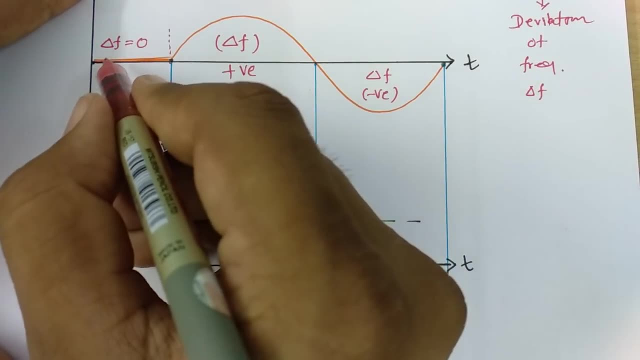 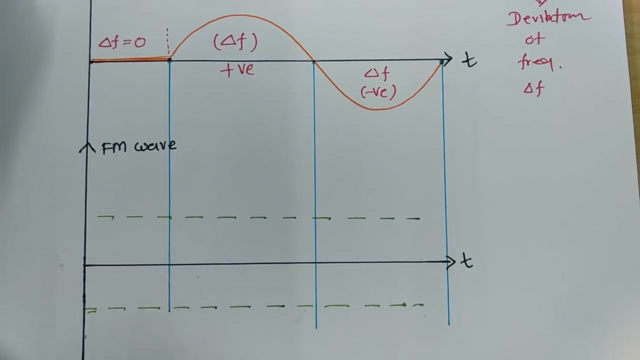 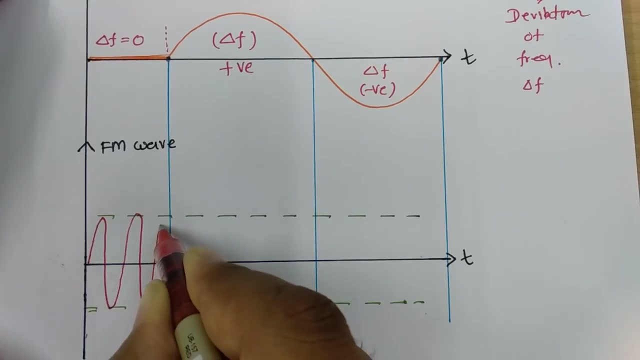 positive or negative frequently. this next equation: 1 1- 1 we have are divisible part as well. this remember Wiring 0. so we will be having a higher evolution of frequency inside of this population and here we will have. So when you plot that wave of frequency modulation over here, carrier signal will be having constant frequency. Why? The reason is deviation of frequency is 0. So as if you plot that you will be finding 0 deviation of frequency. 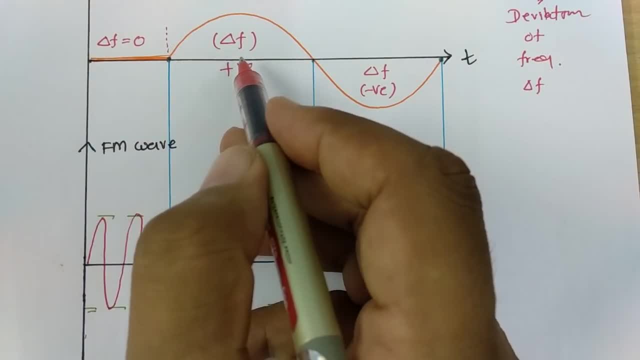 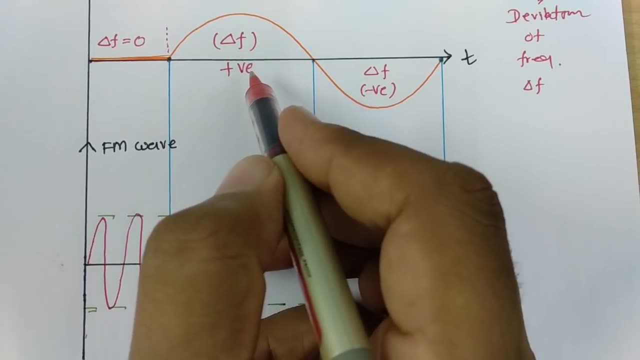 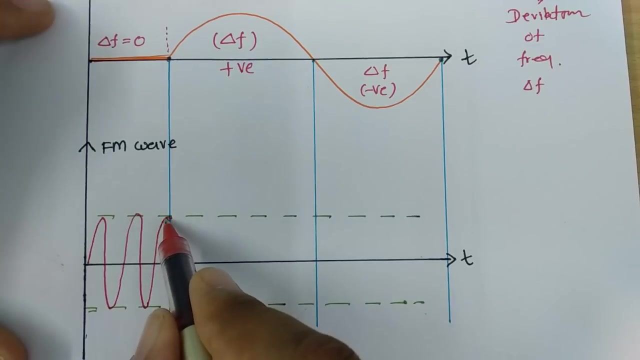 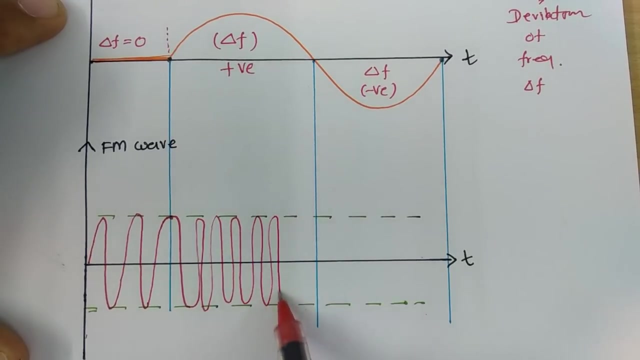 But now, as you see, here we have positive magnitude. So as magnitude is increasing, deviation of frequency is positively increasing. So now you will be finding over here frequency, at this instant it will be maximum. So I am just plotting it, One can see. so here frequency is maximum. 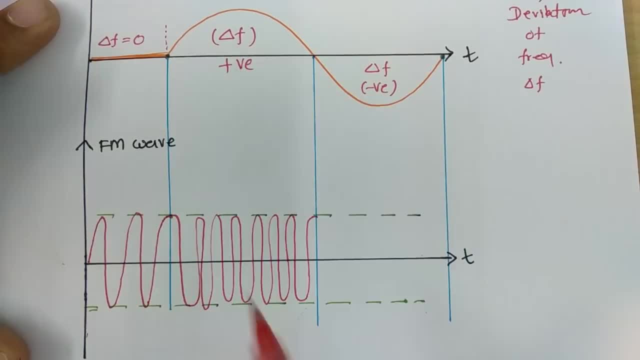 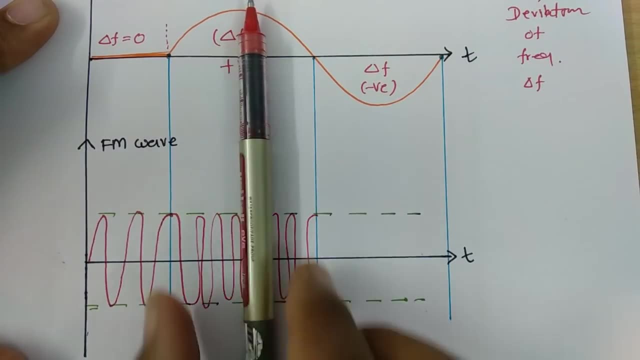 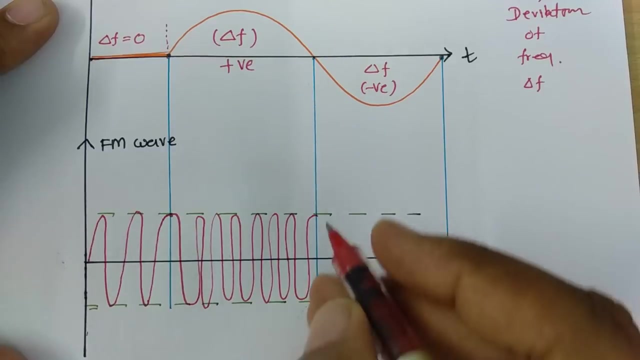 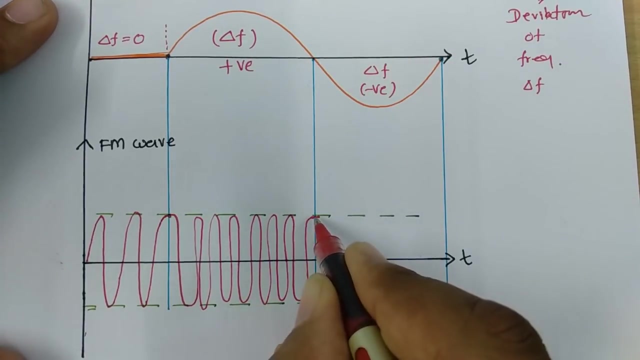 At this instant. Why? The reason is: deviation of frequency is positive and it is maximum over here. Over here it is maximum Now. here negative magnitude is there, So negative deviation of frequency is happening. So one can observe as you go, for negative magnitude of modulating signal, deviation of frequency is getting negative. 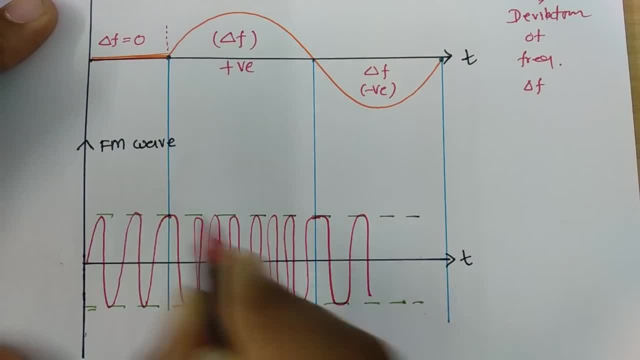 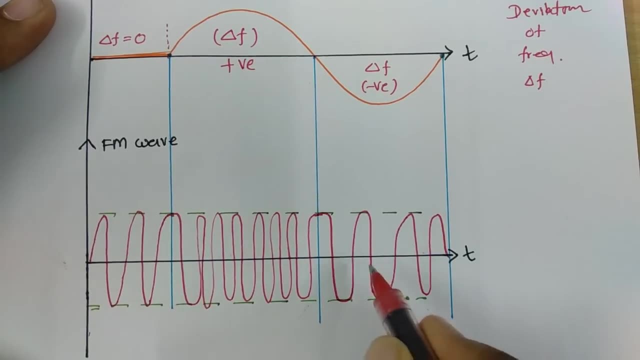 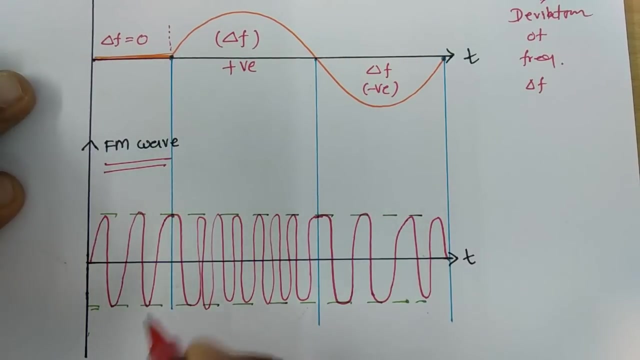 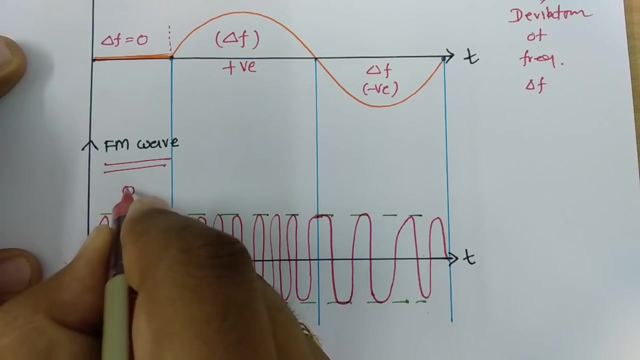 So frequency of modulation. So you will be finding over here frequency is less. So this is how FM wave is responding over here, Like see, as if magnitude of modulating signal is 0. Carrier signal is having constant frequency Over here. magnitude is positive. 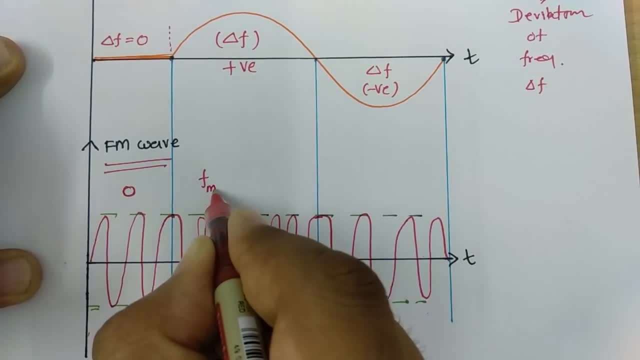 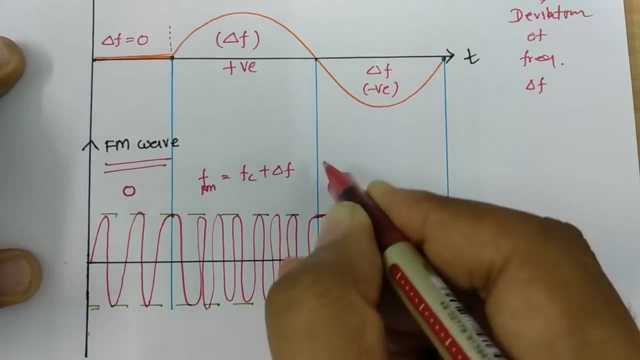 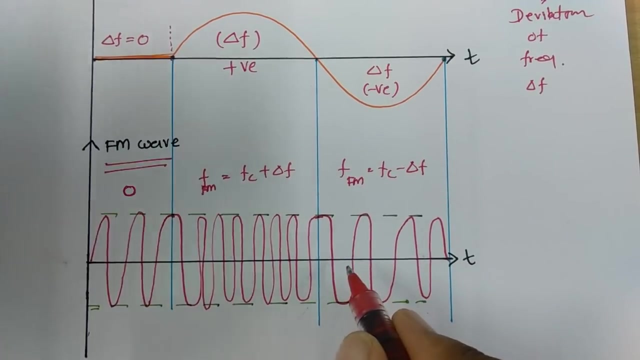 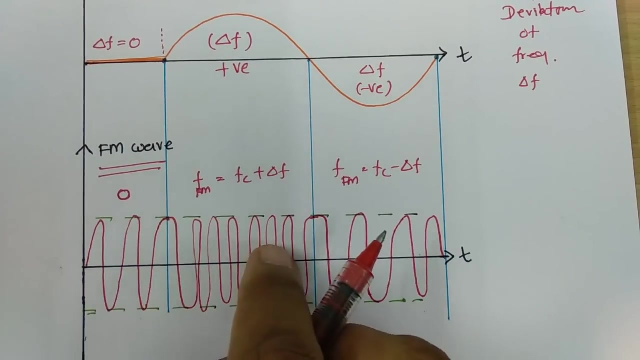 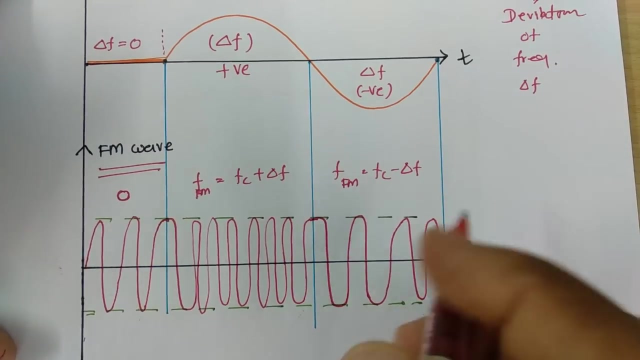 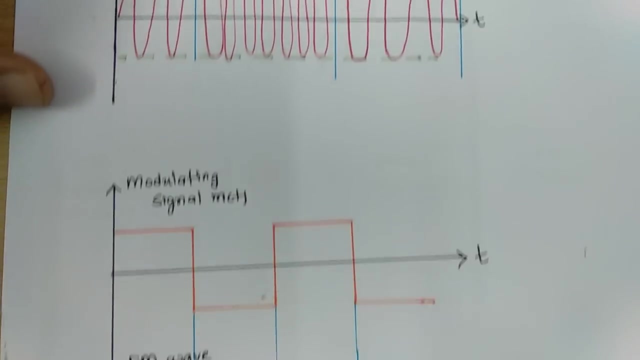 So, So, So. So we will be finding FM frequency that is F C plus delta F and over here frequency of FM that is F C minus delta F. So you can see, over here frequency is less because of separation is more modulation with respect to frequency modulation. now what if you have input that is square wave? 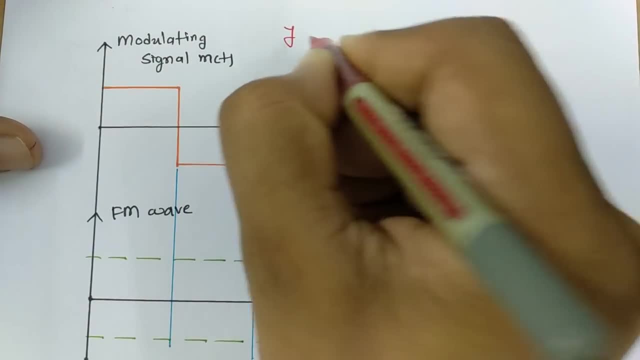 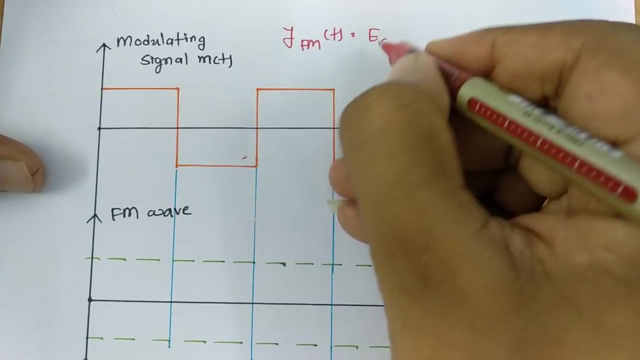 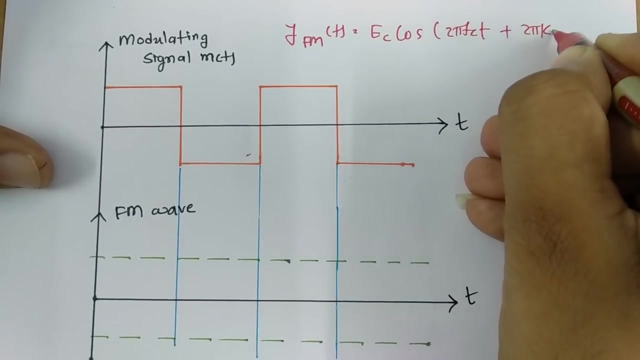 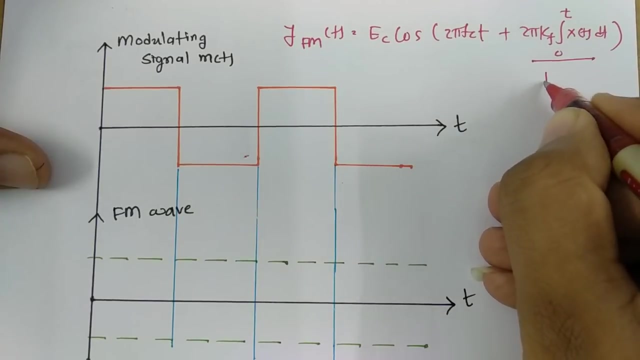 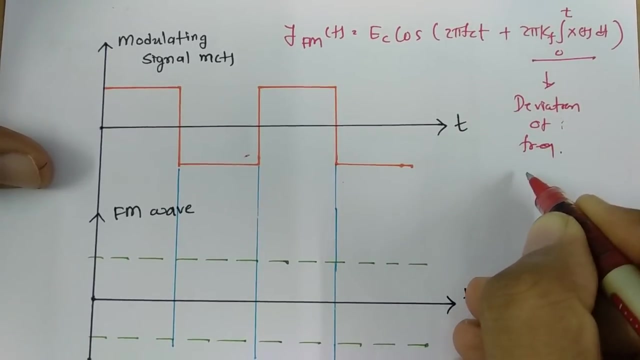 input. so, as i have told you, you have fm signal that is constant ec cos of 2 pi fct plus 2 pi kf integration, xt, dt, where xt integration happens from 0 to t and where this term that will justify deviation of frequency and that deviation of frequency that may be positive or negative.